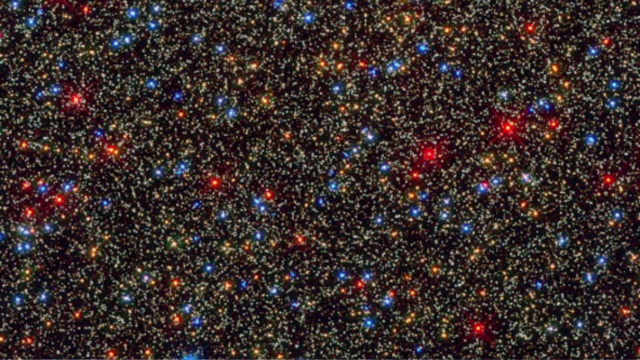 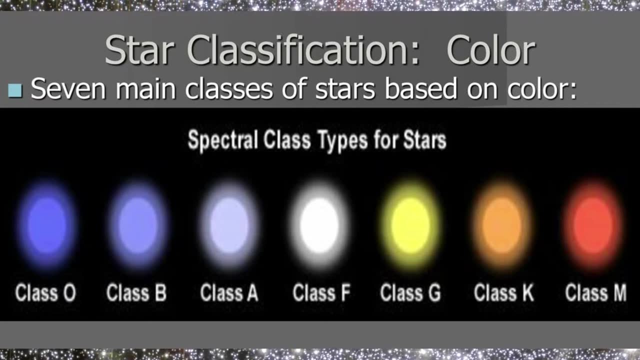 get hotter. The red turns to yellow and then white and eventually bright blue. The same way, it turns out that blue stars are really hot and classified as O type stars, whereas cooler red stars are placed in the M class. There are other types beyond the original: O, B, A, F, G, K, M, Q. example is for: 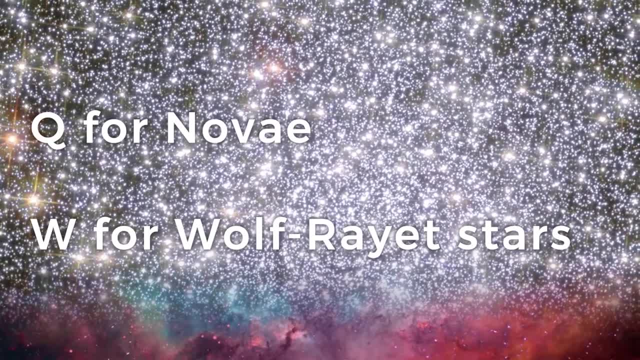 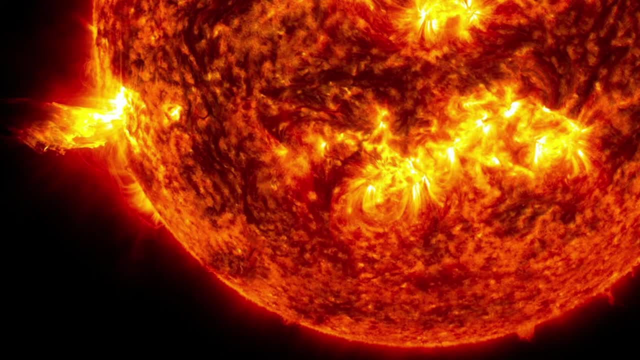 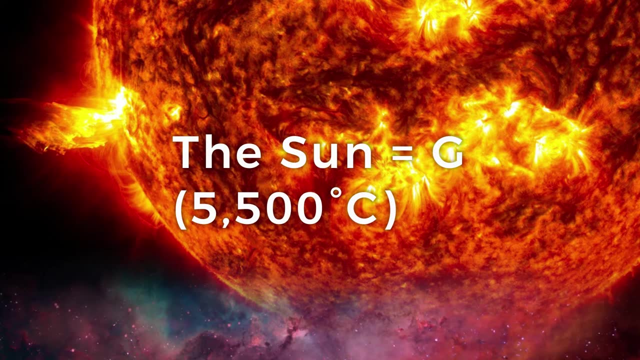 a Nova W is for a Wolf-Rayet star, but they're not encountered frequently and we're not including those today. Now Sun: We think of it as yellow. therefore, it's not surprising to discover it's classed as a G star with a temperature of around 5,500 degrees C on its surface. The table you can see lists the. 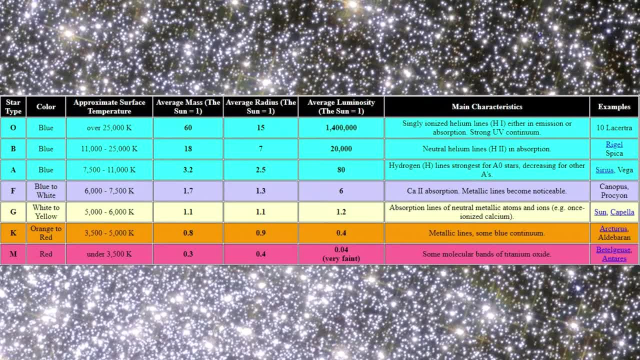 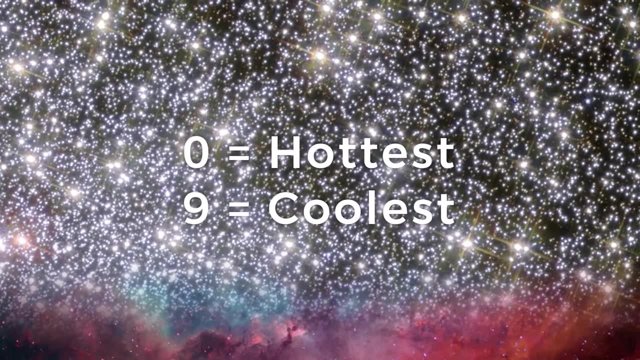 different stars according to their temperatures and colors. but stars can be more accurately categorized under the system by the addition of the number 0 to 9.. Beginning with a 0 is the hottest and 9 is the coolest. so, for example, a G2 star is hotter than G7 star, but cooler than a G0. 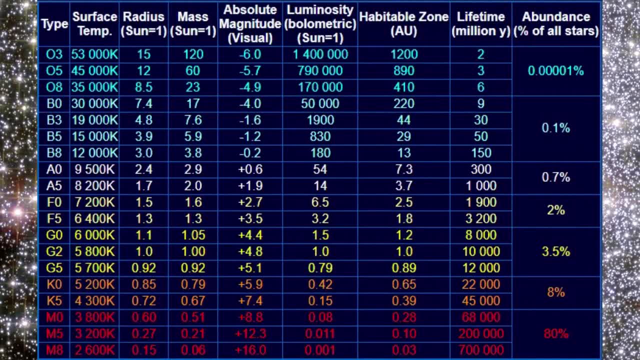 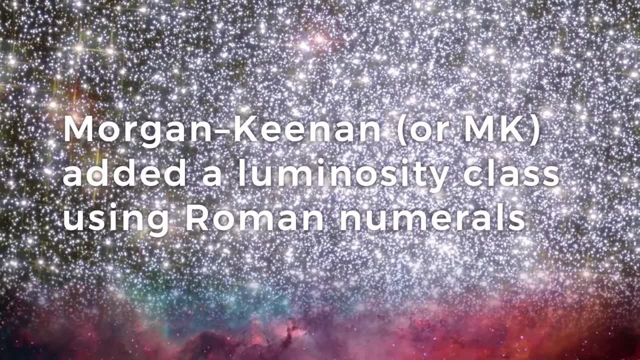 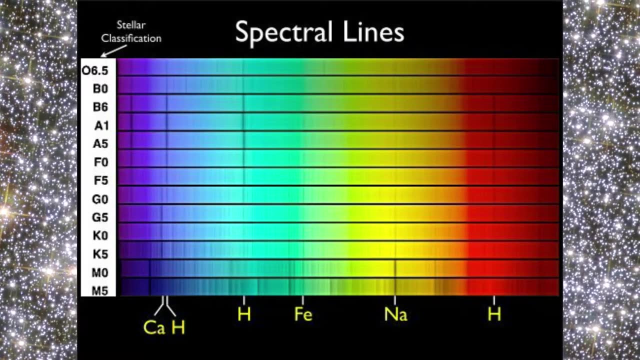 similarly, a B9 is cooler than the B4.. In the MK system, Illuminosity class is added to the spectral class using Roman numerals based on the width of certain absorption lines in the star spectrum. Have a look at our video on the electromagnetic spectrum for more details on that, and this varies greatly. 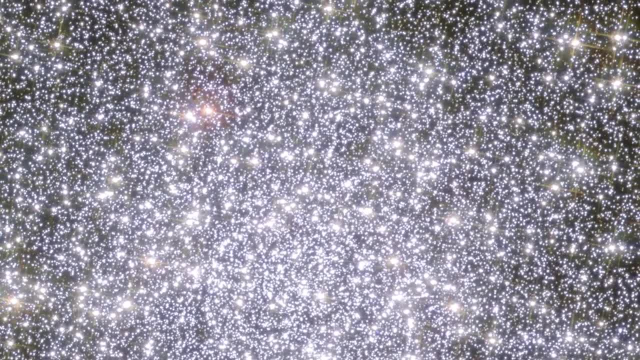 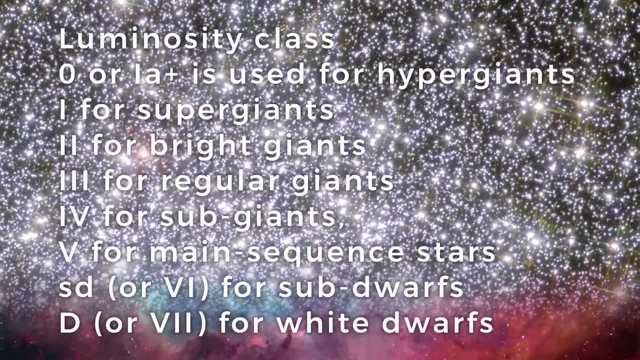 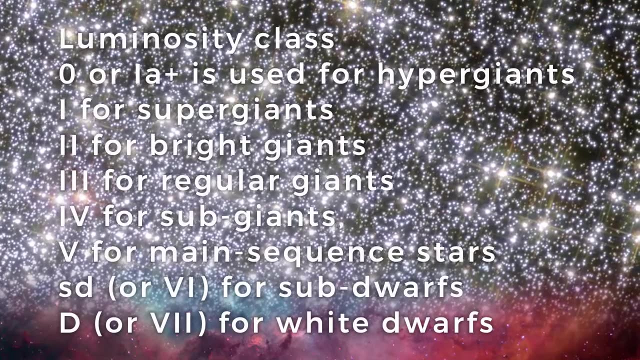 with a density in the atmosphere. so distinguishes giant stars from dwarfs. Illuminosity class 0 is used for Hyper Giants, class 1 for super Giants, 2. Pi bright giants, three for regular giants, four for sub giants, five for main sequence stars, such as: 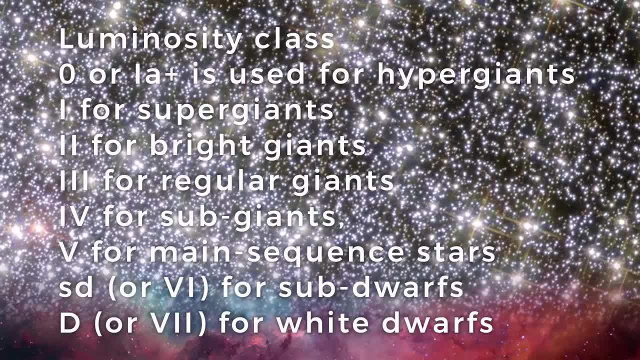 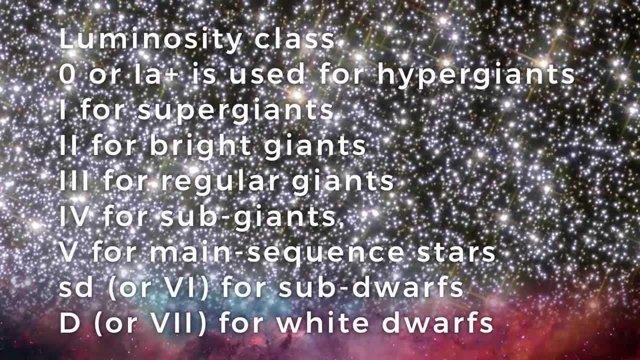 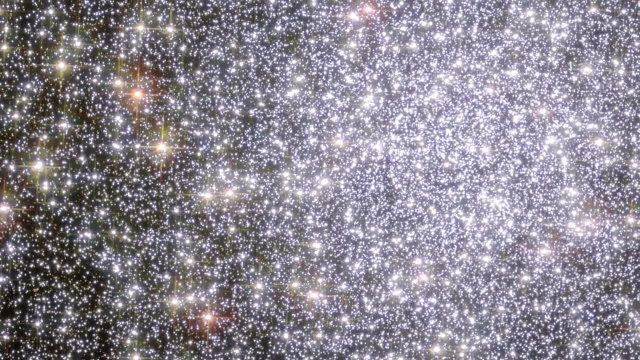 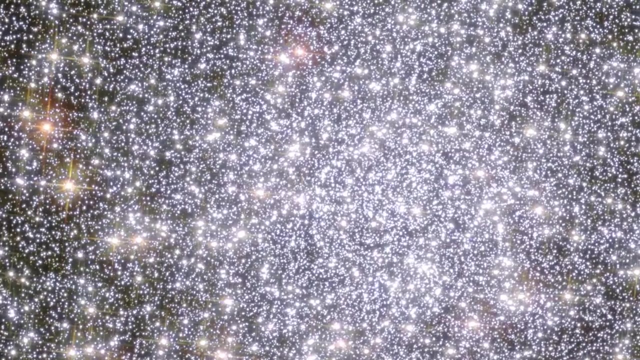 our sun, class six for sub dwarfs and class seven for white dwarfs. sometimes those last two classes six can be classed as sd and seven can be classed as d, so the full spectral class of our star is a g25, indicating a main sequence star with a surface temperature, as we say, around five thousand. 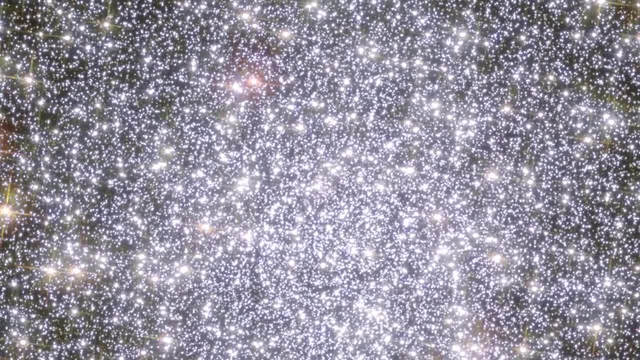 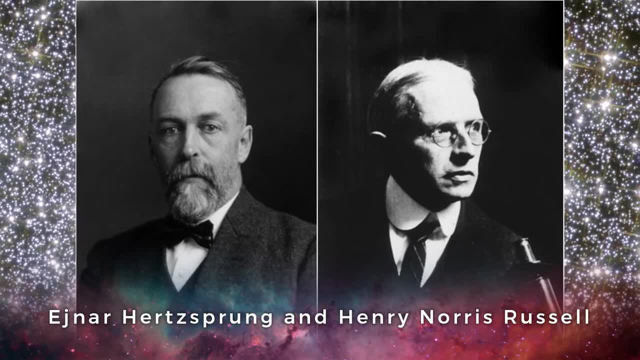 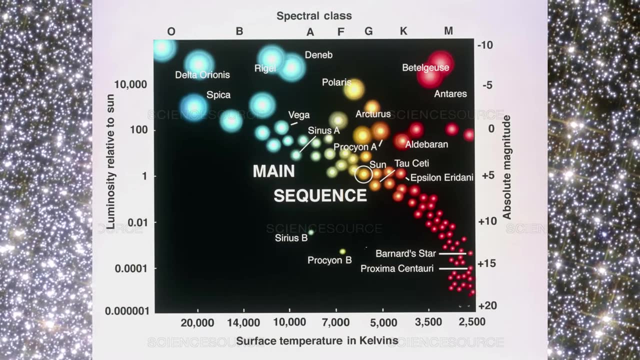 five hundred degrees c, five thousand eight hundred degrees k. the hr diagram devised by henya hertzsprung and henry norris russell, otherwise known as the hertzsprung russell diagram, simply puts all this information into a graphical format and, whilst it can be confusing, 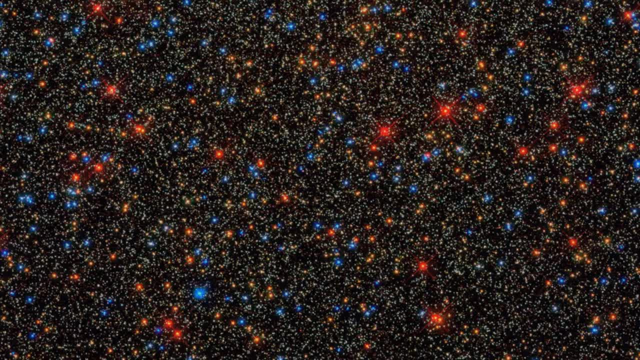 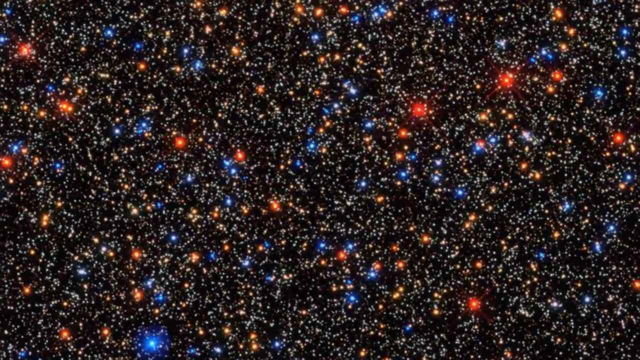 at first. it's actually confusing at the same time. it's actually confusing at the same time, quite easy to understand when you understand where the information comes from, which i hope you do. now we can see on the diagram the line that runs from the top left down to the bottom right. this is what 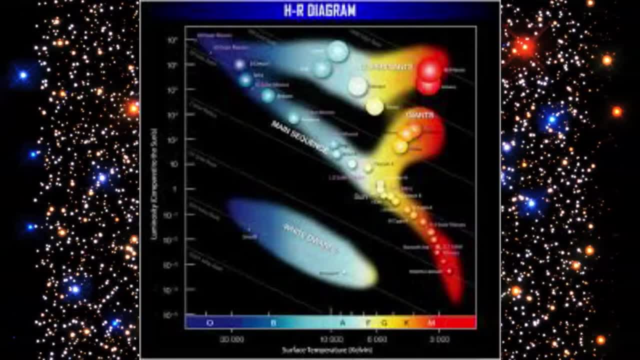 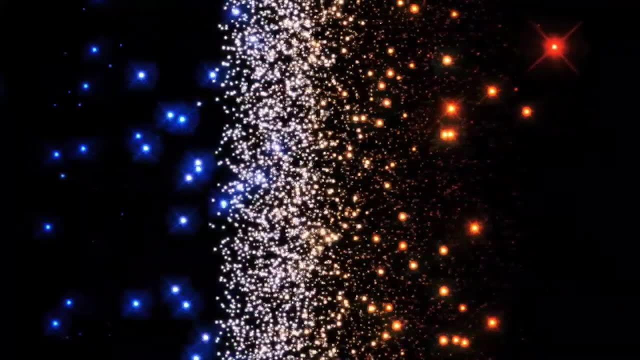 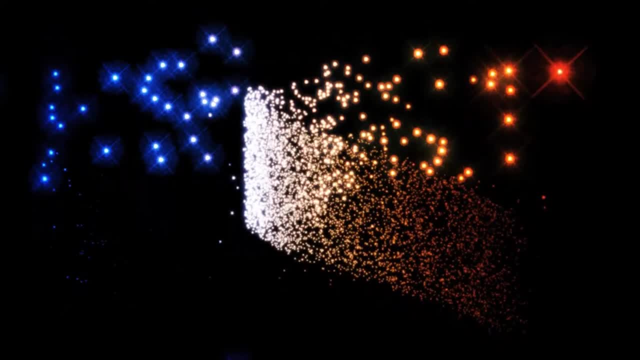 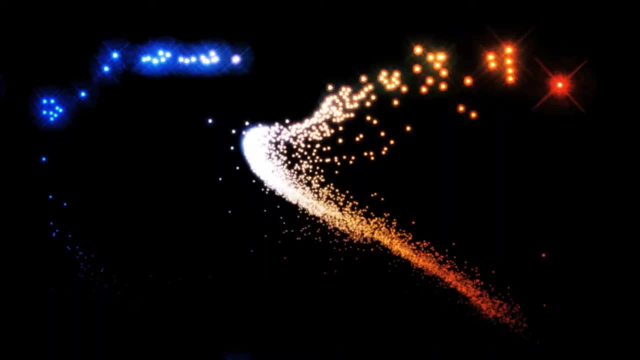 giants and so on. so it isn't that hard. luminosity scale is on the right, the surface temperature in kelvin is along the bottom and the absolute magnitude is up on the left hand side. and if you want to look at magnitude, we have another video on stellar magnitude as well. 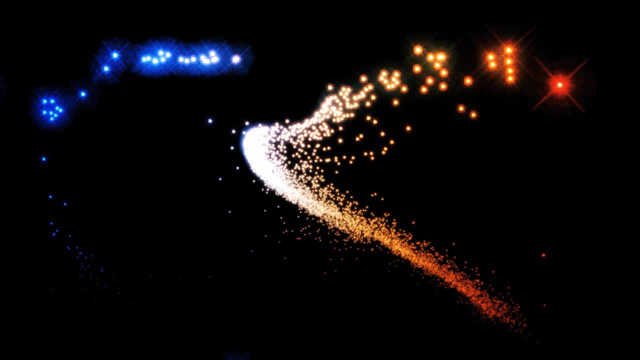 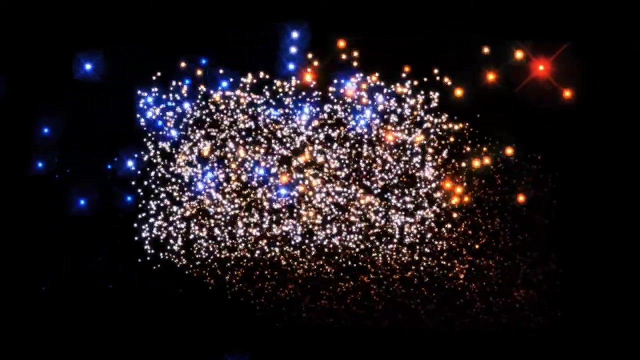 there are a few other methods of classification, such as the sechi classes, the draper system, an earlier harvard system and the mount wilson classes, but none of these are as all-encompassing as the mk and the hr systems. well, i hope you enjoyed that little look at how we classify stars. 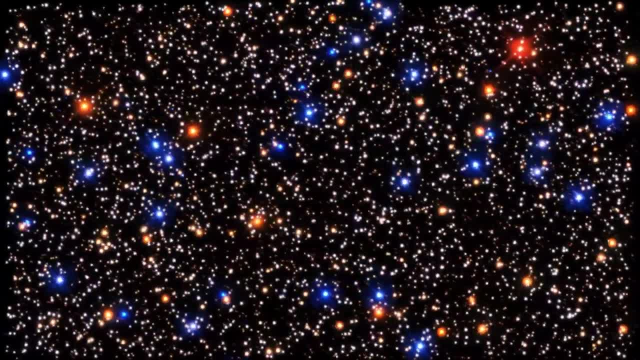 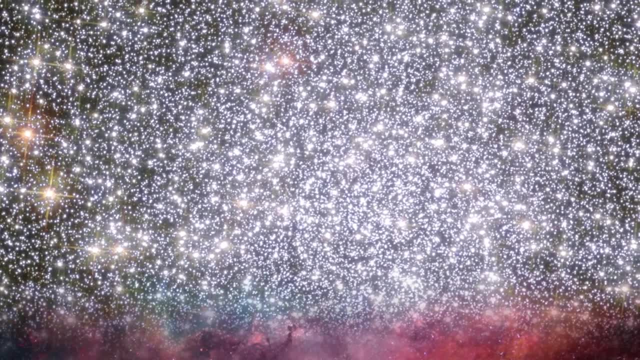 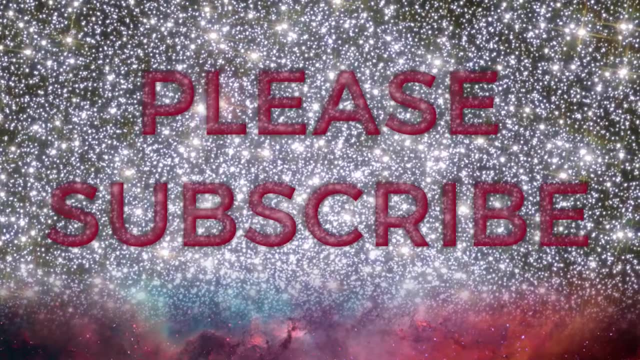 and maybe understand a little more when you read about, say, a g2v star or so on. well, clear nights, happy stargazing, and see you next time. thank you, and please remember, do subscribe. subscribers mean an awful lot to me. it shows that people are interested in what i am doing. and i will see you in the next video. 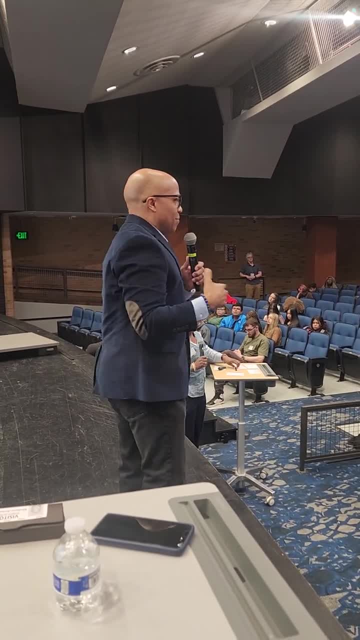 I'm trying to wave my hand and say: hey, we've got a new position here, a new assignment. It might not have been the most glamorous one, but I just raised my hand and did it just because it was something new and interesting. 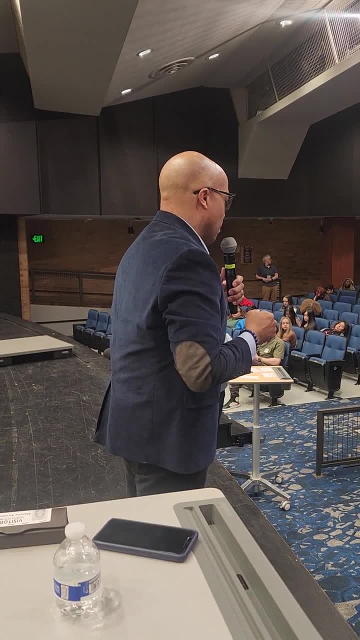 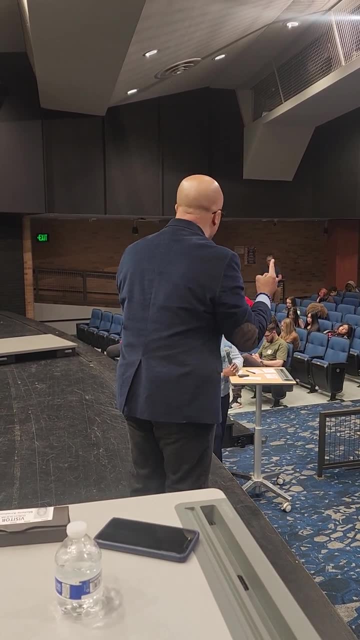 So over the course of my career I basically was in a position. I worked so many different pieces of the organization. I was never a subject matter expert at one part of the job, but by the time I actually became chief I had worked basically every position within the organization.